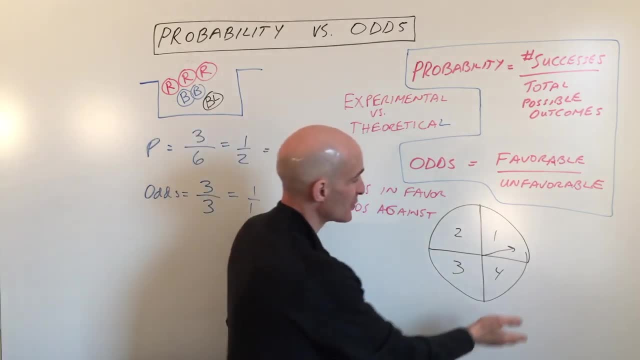 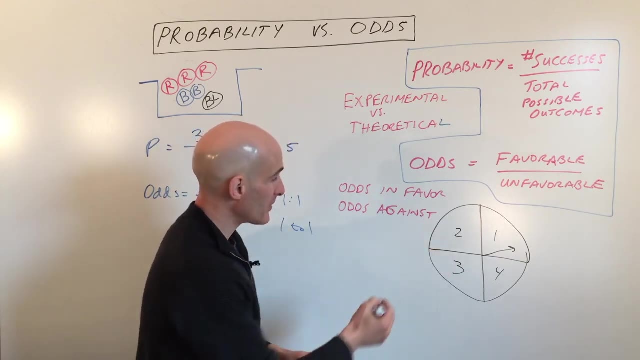 Let's look at the spinner over here. Okay, say, for example, the spinner, we're going to spin it, and we say, well, what's the probability that I land on two? Well, there's only one, two. okay, these regions are, all you know, the same size and shape. So 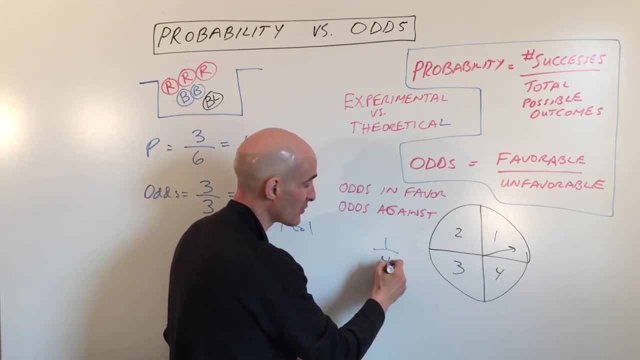 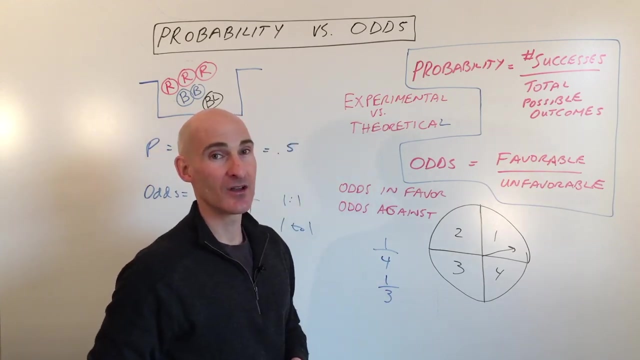 there's one chance of landing on two divided by four possible outcomes, the probability is going to be one- fourth. But if we said, what are the odds that you land on two? Well, one chance of landing on two to three chances of not landing on two. the odds would be one to three. Okay. 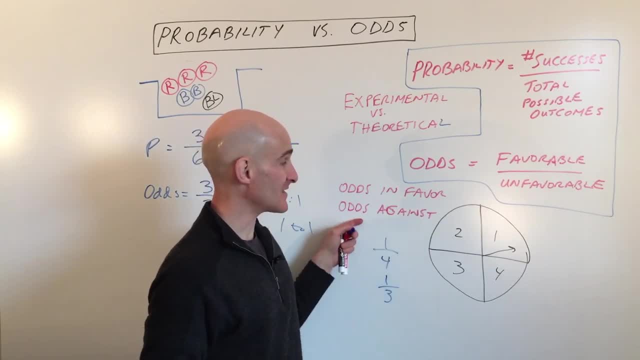 now let's switch it up a little bit. Let's say we want to find out what are the odds against landing on the number two. So now the odds against means we don't want to land on two. So what are the chances that we don't? 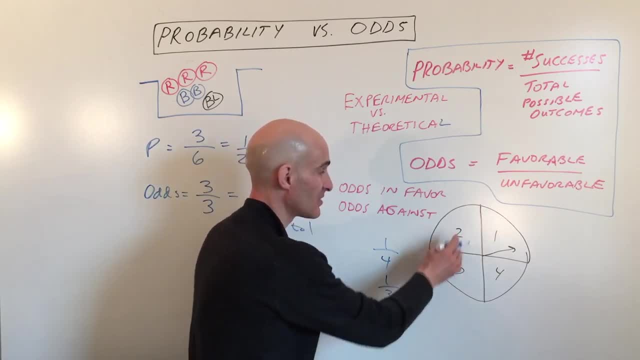 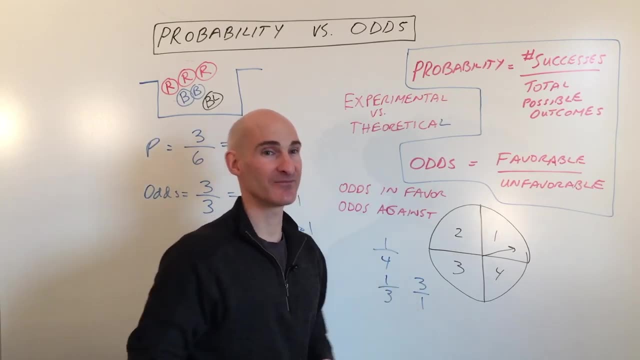 land on two. Well, there's three non-twos to one, two. So the odds against would be three to one. Notice, it's the reciprocal of the one that we did, odds in favor. So odds in favor is what you want. 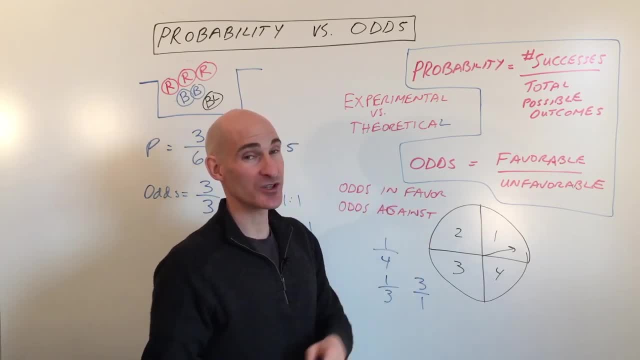 to what you don't want. Odds against is what you don't want to what you do want. Okay Now, experimental versus theoretical probability: what's the difference? Well, say for example: we run an experiment, right, We spin. 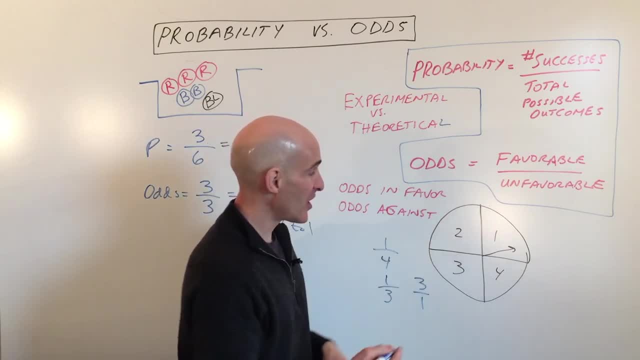 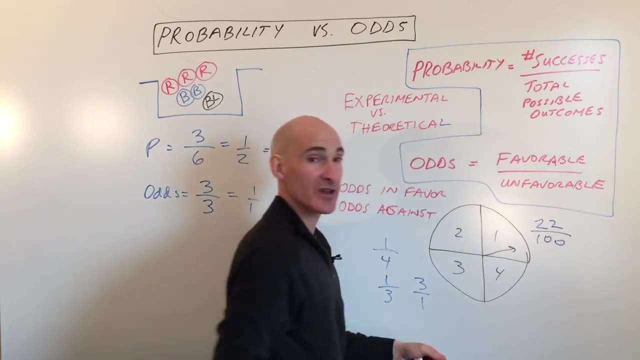 this spinner 100 times and out of those 100 times, let's say the number two comes up 22 times. Okay, so the experimental probability would be 22 out of 100 trials. That's the probability and you could reduce it down. It would reduce down to 11,. 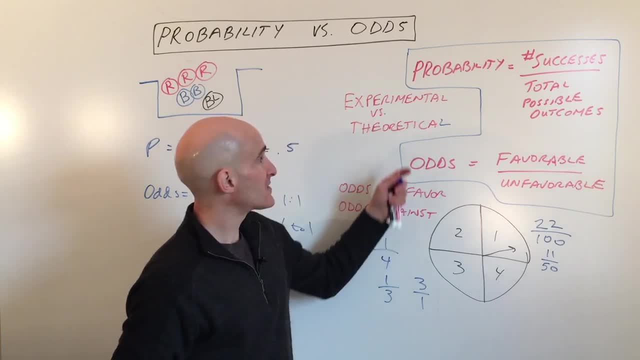 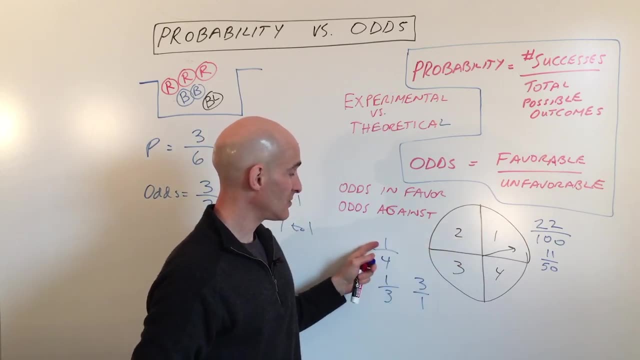 50th right. Good, divide them both by two. But what's the theoretical? in theory, What's the probability that we land on two on to well, one chance of landing on two out of four possible things that could occur. right so experimental. you just think you're running an experiment. 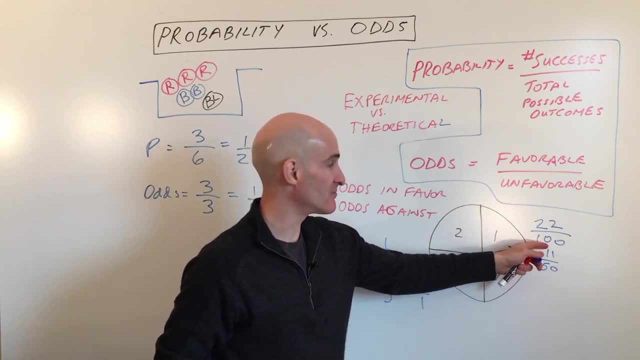 you're running trials, you know you do it a hundred times or twenty times, or a thousand times, and you count how many successes, how many things occur that you're interested in having happen, out of the total trials. and that's your experimental probability now, as the number of trials go up. okay, assuming.